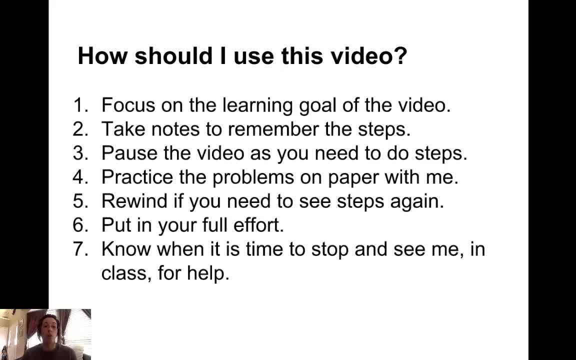 much as I can and you need to save that work, bring it to class tomorrow, jot some questions down on the side so that you and I can sit down and talk about your math. So let's look at addition first. Our strategies for 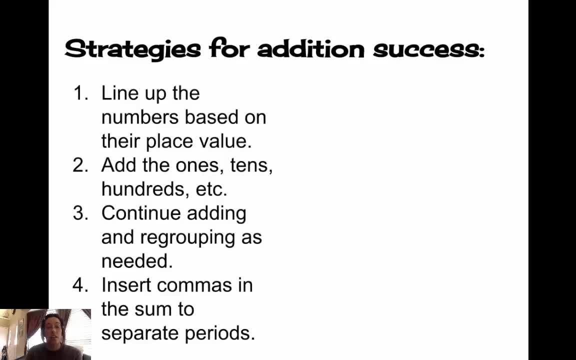 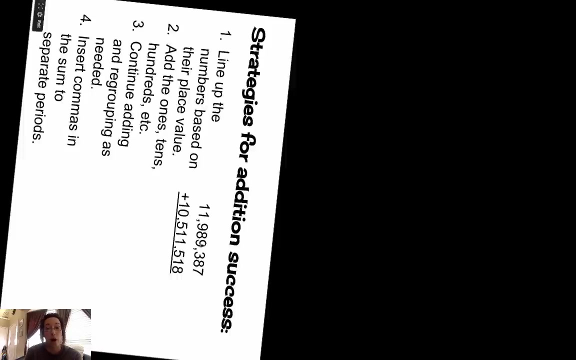 addition success. First you need to line up the numbers based on their place value. You add the ones, the tens, the hundreds, the thousands, and so on. Continue adding and regrouping as you go and then insert the commas into the sum to separate the periods. So let's look at some problems here. Our first problem is eleven million nine hundred eighty nine thousand three hundred eighty seven plus 10 million five hundred eleven thousand five hundred eighteen. It looks big, but if you follow the steps, you'll do well solving this problem. Okay so let's go ahead and get our scratch paper out, and let's work this problem together. 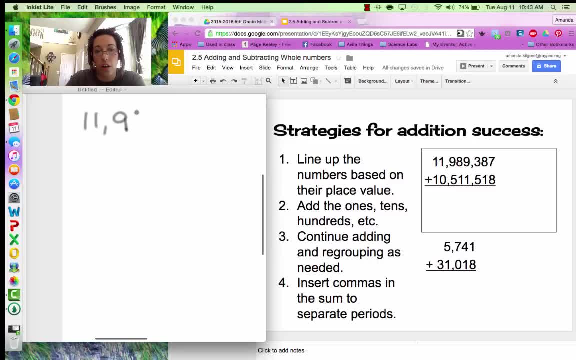 We've got 11,000,989,387. We are adding ten million nine hundred eighty nine thousand three hundred eighty seven. approaches theém and so on. 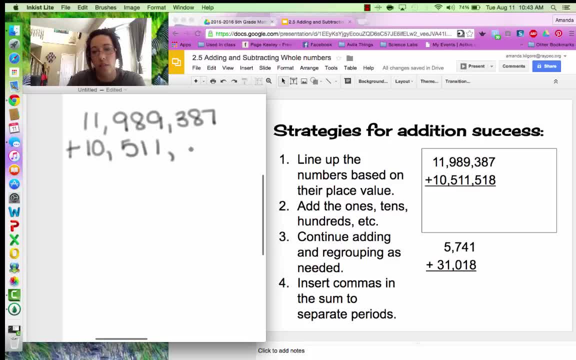 511,518. Okay, so when I look at this problem, I look at step number one and line up the numbers based on their place value. I've got my ones, tens, hundreds, thousands, ten thousands, hundred thousands, millions, and ten millions. So I start adding at the ones place. Seven plus eight is 15. That's more than nine, so we have to regroup. We put our five down here and carry the one up here. Eight plus one is nine, plus one more is ten. So again, we have to regroup. Five plus three is eight, plus one is nine. Nine plus one is ten, so zero down here. Regroup. Eight plus one is nine, plus one is ten. 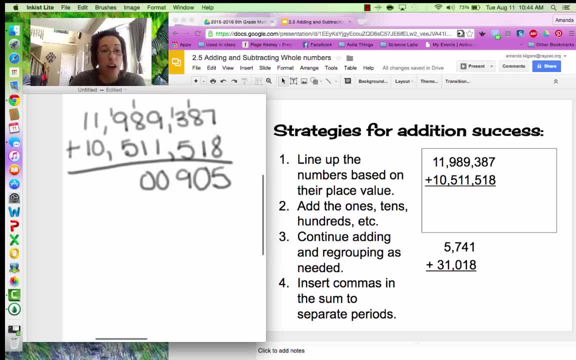 Zero. Regroup. Nine plus five is 14, plus one is 15. So again, regroup. One plus zero is one, plus one is two. 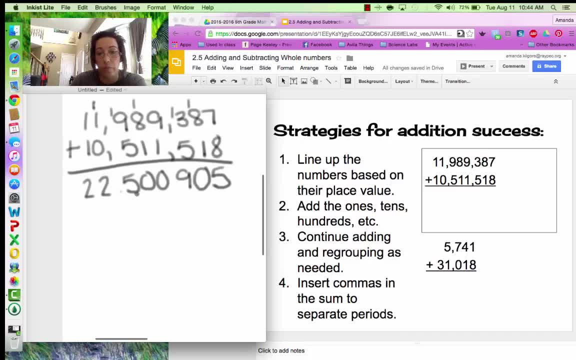 One plus one is two. So we've added and regrouped as needed. Now we have to insert commas into this sum or answer to separate the periods. We start at the ones place, go one, two, three spaces, comma. 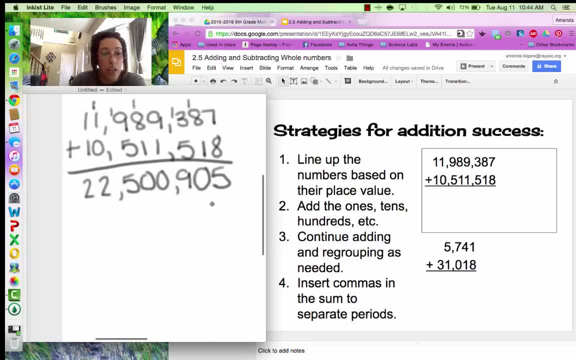 And we end up with 22,500,905. 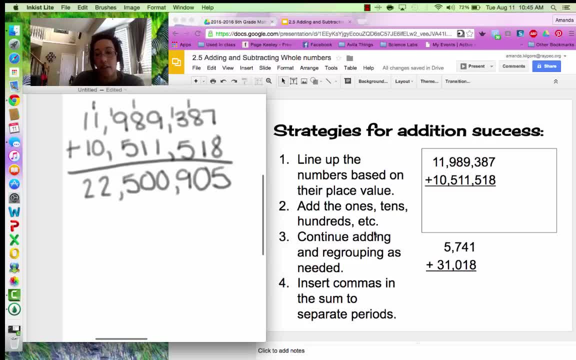 Okay, so let's look at this next example. Notice that in this problem, we've got 5,741, but we're adding to it 31,000, so we have to be very careful and know that our place value starts at the ones place. So 5,741. 31. 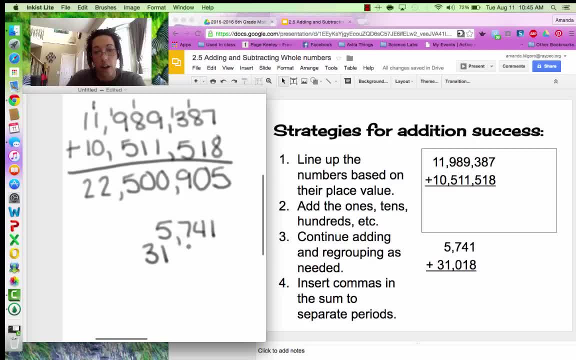 To that, we are adding 31,018. 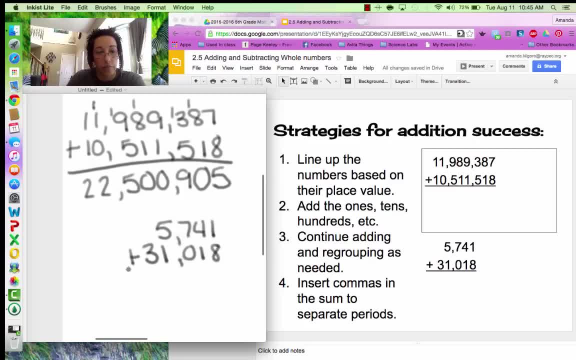 Problem is set up here. Let's look at this. 1 plus 8 is 9. 4 plus 1 is 5. 7 plus 0 is 7. 5 plus 1 is 6. Nothing plus 3 is 3. Go back and put our angle here. 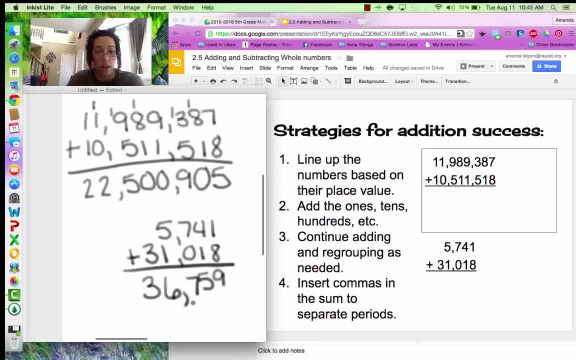 commas in. One, two, three, comma, 36,759. I hope that this has helped refresh your adding 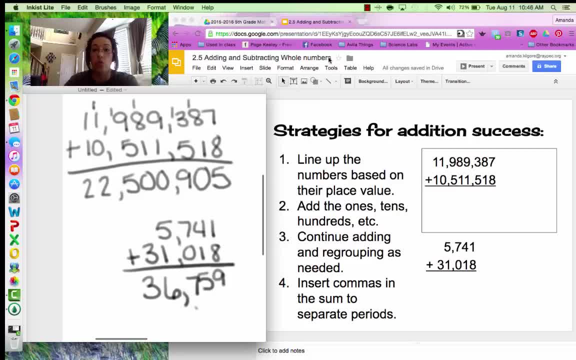 large number skills. We're going to move on to subtracting. 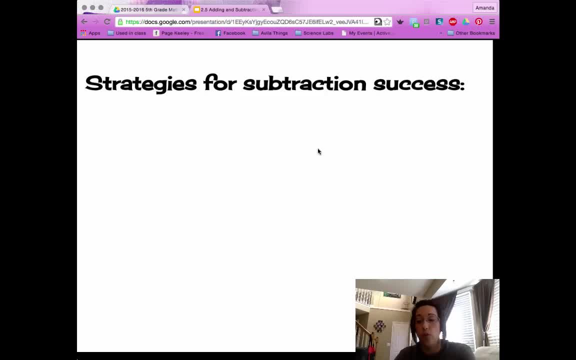 Okay, so now we're looking at our strategies for subtraction success. Let's look at the list of steps. First, we're going to line up the numbers based on their place value again. We're going to subtract the ones, tens, hundreds, thousands, and so on. Continue subtracting and regrouping as we need to, and then inserting commas into the sum to separate the periods. Similar process to addition, only we're subtracting this time. So let's look at our problems here and get them set up. 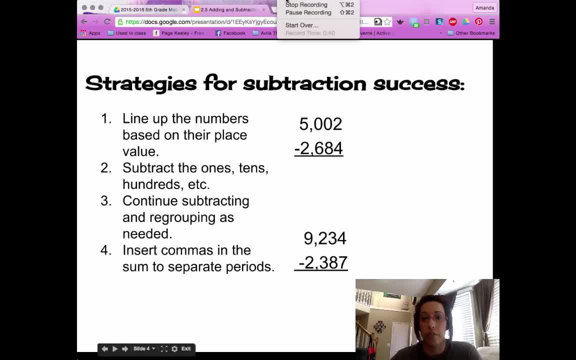 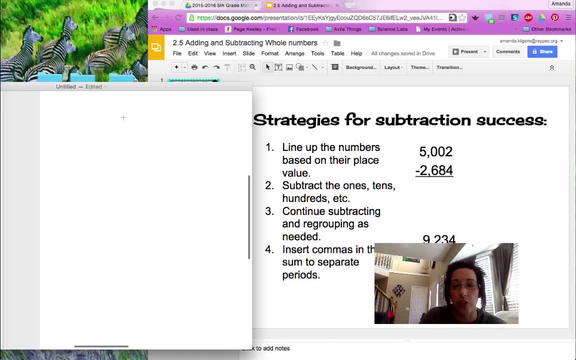 Okay, let's go ahead and set up these subtraction problems on our scratch paper. We have 5,002, and we are subtracting 2,684. So let's look at this problem. In the ones place, that's where we always start. We're going to subtract the ones, tens, hundreds, thousands, and so on. So let's look at this problem. In the ones place, that's where we always start. So let's look at this problem. 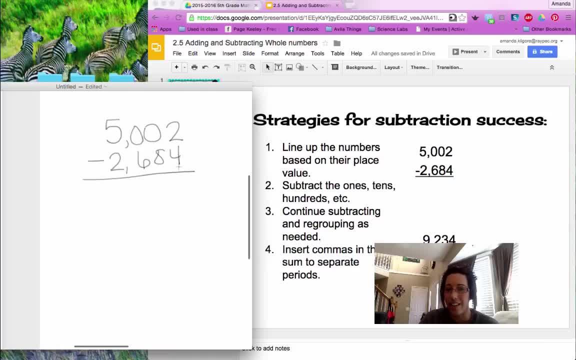 We have 2, subtract 4. Now, if I have 2, I can't give 4 away. So I have to go ahead and regroup so that I've got enough to subtract from. But we've got a 0 here and a 0 here, so I've got to regroup across some 0s. Our 5 is going to become a 4 because we're borrowing 1,000. We're going to add it to the hundreds place, but we need to borrow 1 from that, so it becomes a 9. We're going to add a 10 either way, but 아u got to borrow 1st place, so we could borrow 1 from that, too, so it also becomes a 9. And then this 2 becomes a 12. So 12 subtract 4 is 8. 9 subtract 8 is 1. 9 subtract 6 is 3, and then 4 subtract 2 is 2. Go back to the ones place, count 3 over. 1, 2, 3, put your comma in to separate those 我們 the periods. There is the first problem. Let's look at the second one. We have 9,234. 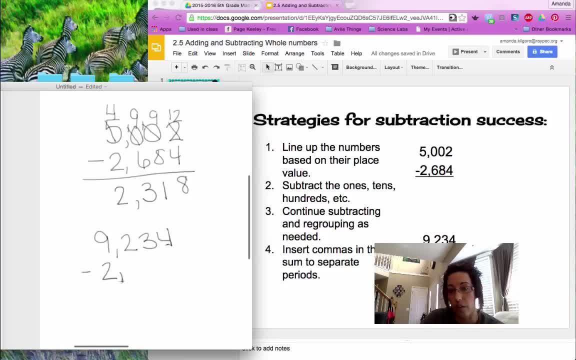 We are subtracting 2,387. So I noticed right away in our ones place, we are going to have to regroup. So we are going to borrow 1 from the 10s. Our 3 becomes a 2. Our 4 becomes a 14. 14 subtract 7 is 7. We have got a 2 and need to subtract 8. So we have to regroup again. This becomes a 1. Our 2 becomes a 12. 12 subtract 8 is 4. We have to regroup again. So 9,234.